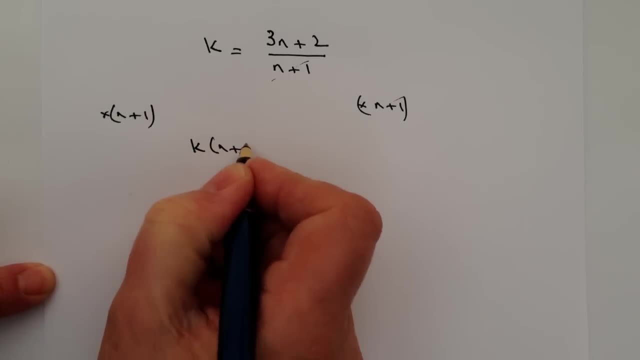 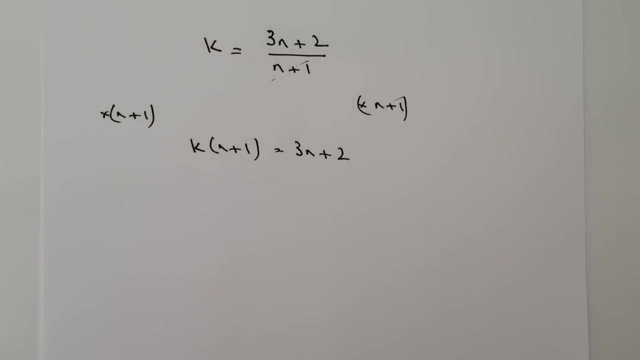 itself becomes K times N plus 1 equals 3N plus 1.. Okay, I hope that's alright with you. If you're not sure about that, if you have a look at some of the other videos on the playlist, that will give you a little bit more help. 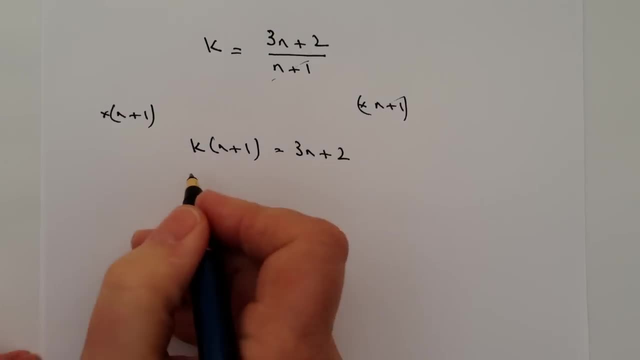 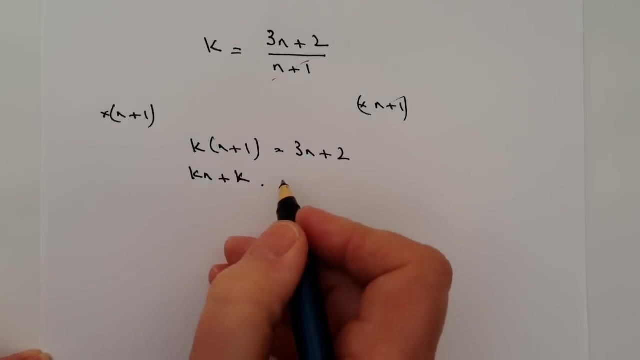 Okay. so the next thing is we need to multiply out the brackets. So I'm going to multiply out the left hand side as KN plus K. So remember that K times N is KN and K times plus 1 is going to be plus 1K, which you would just write as K on its own, And that equals 3N plus 1.. 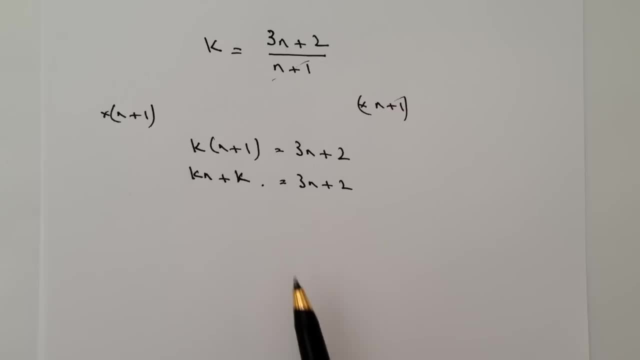 So I'm going to multiply that by 3N plus 2.. And then really, it's just a matter of getting the N terms together on one side and everything else on the other. So what I'm going to do is I'm going to get this 3N over towards the left hand side. So 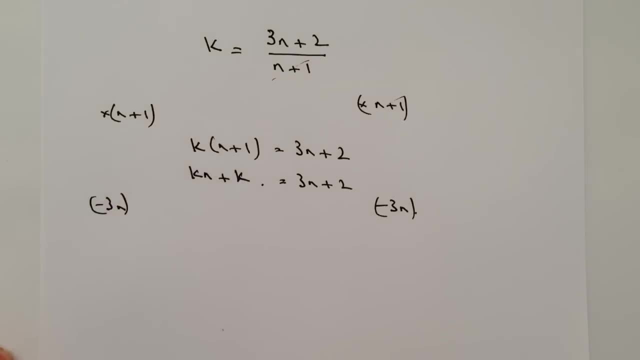 if I do that by minusing 3N over here and minusing 3N over here, it means then I end up with KN minus 3N plus 1.. So I've got 3N plus K equals 2.. Alright, then I need to get this K over towards my right. 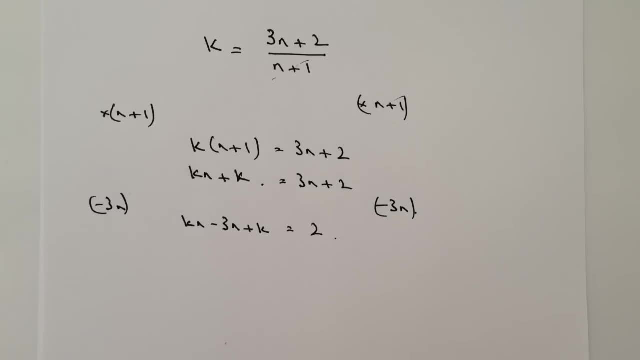 hand side here. So the way I'm going to do that is I'm going to minus K from both sides, And that's going to be great because I'll end up then with a situation where I've got both of my N terms on the left hand side and everything else to minus. 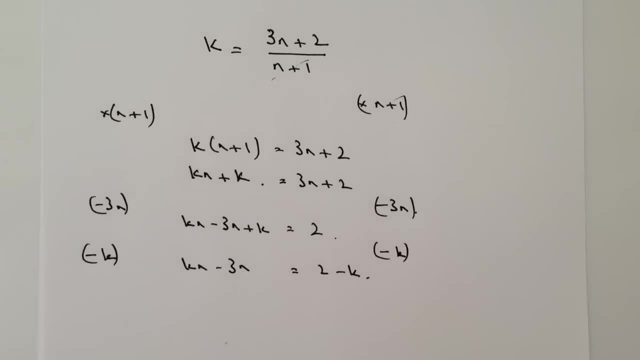 to minus k on the right hand side. OK, so the easiest way of dealing with this is then factorising my n terms, because then I can isolate n on its own as being n times k minus 3 equals 2 minus k, And then, because this is a multiplication of n, I can then just 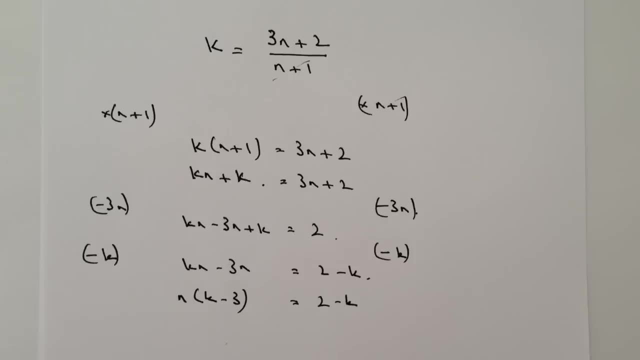 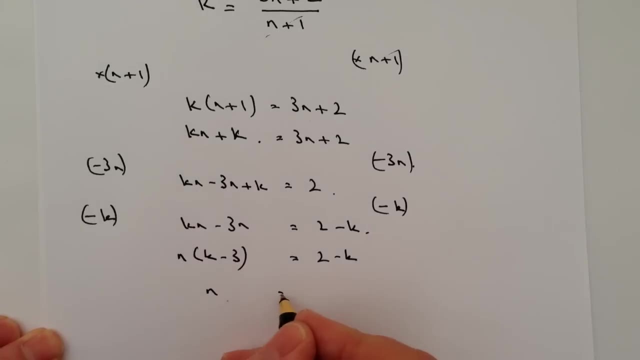 simply divide through by k minus 3.. So what I end up with at the end of it is just an expression for n of 2 minus k divided by k minus 3. And that would be the answer to this particular question. However,